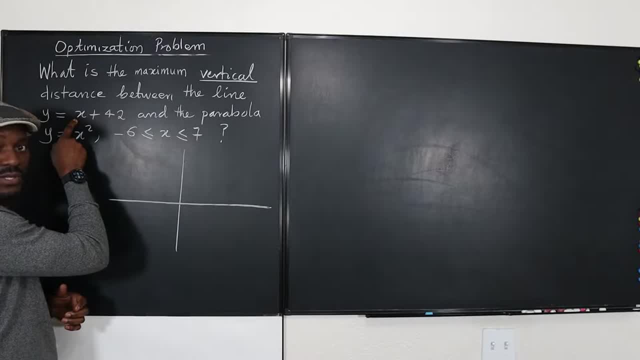 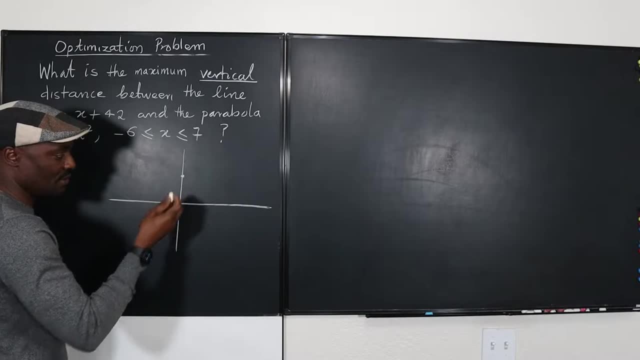 looks like this: a straight line. Well, it has a positive slope And the y-intercept is positive, so the y-intercept has to be somewhere here. So let me say: this is the point where it's 42,. okay, And because it's a positive slope, so I can say something. 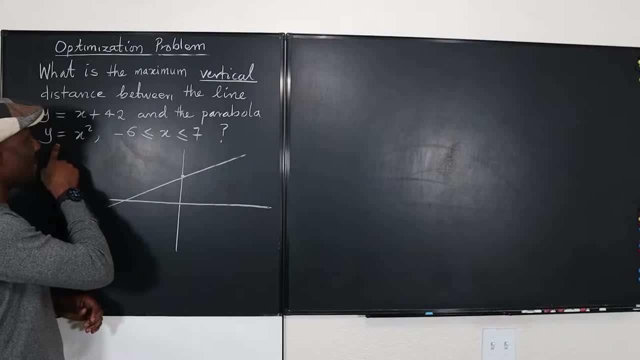 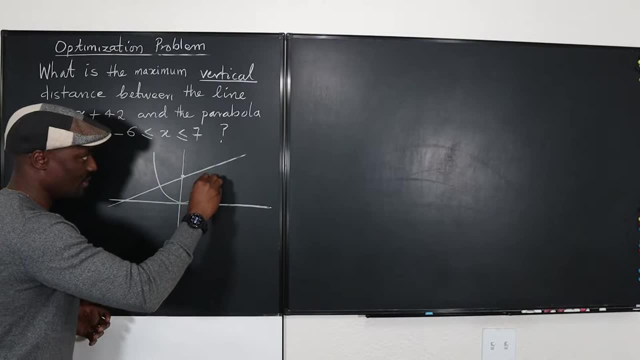 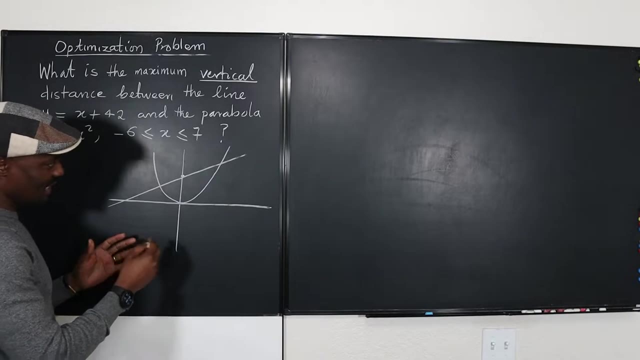 like this. okay, Now the other graph is the graph of y equals x squared, And the graph of y equals x squared is just the graph of the parabola, something like this: So you can see that the distance between this function. 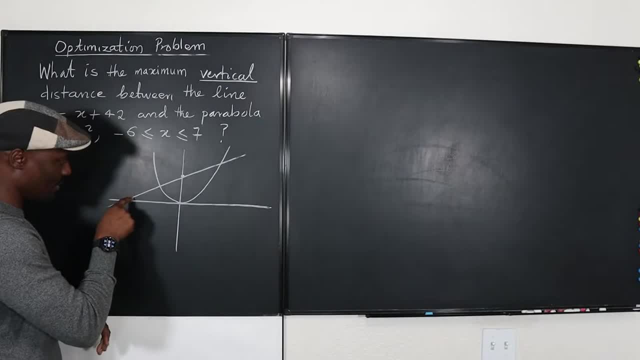 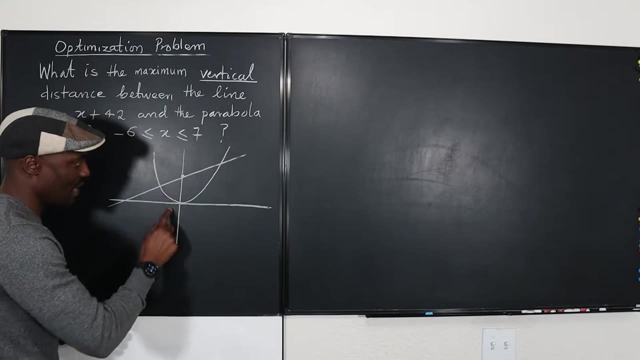 and this curve can be measured from anywhere. You can measure from here to here. There'll be a horizontal line, But we're referring to the vertical distance, So it has to be that it's as if you get a ruler and then you place a ruler here and you just draw. 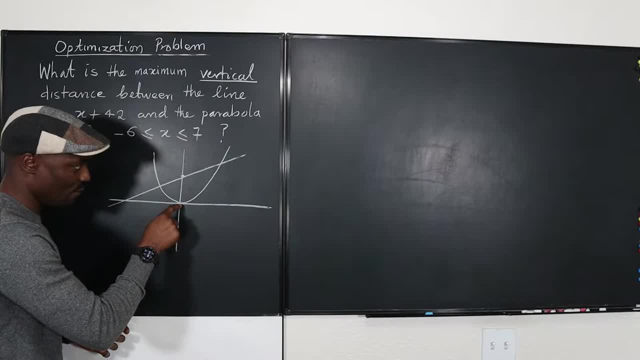 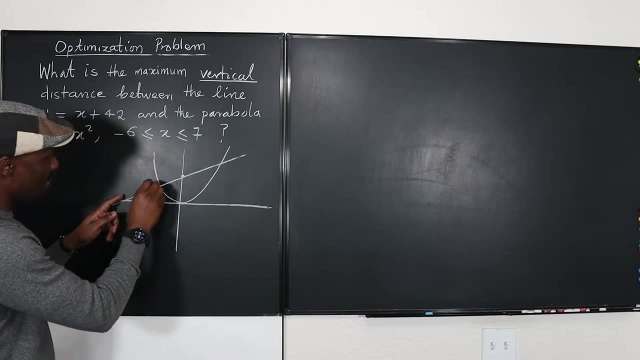 a vertical line, So this is a good candidate. The length of this line will be the distance between the two, but we're looking for where the distance is the greatest. Now it's possible that, if you See, If you draw it up like this, then this distance would be a huge distance. But the question 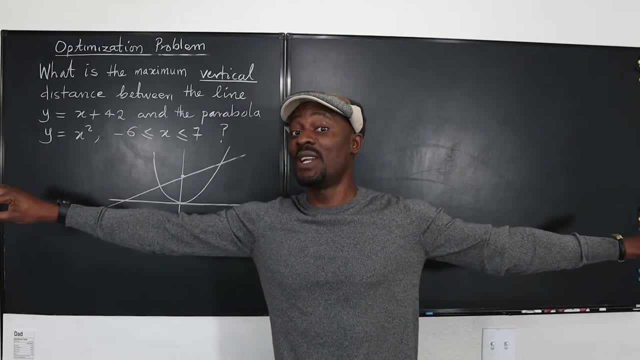 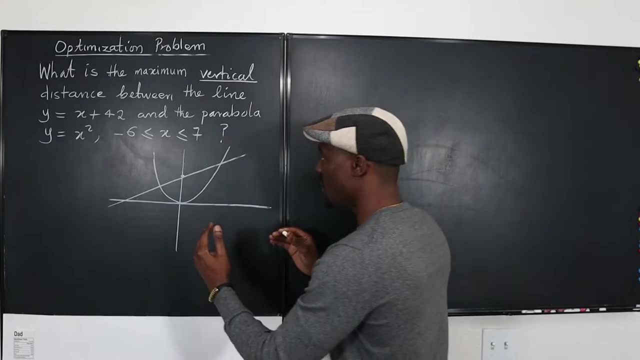 has said: no, no, no, no, Don't go all the way to the left or all the way to the right. You want to stay between negative six and seven. So we want to stay between negative six and seven. So somewhere around here- well, we don't know- It's possible for you to find. 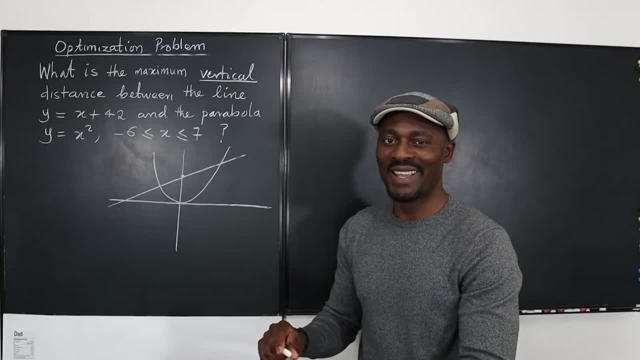 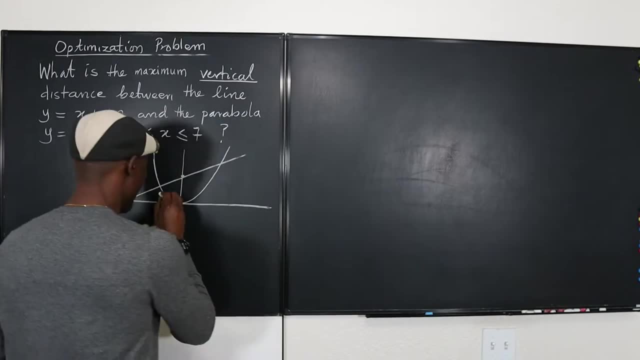 out where it is. Maybe I should just tell you, okay, The point where these two graphs meet. those are actually the points negative six and seven. So we're saying that this point will be negative six and this point here will be at seven. 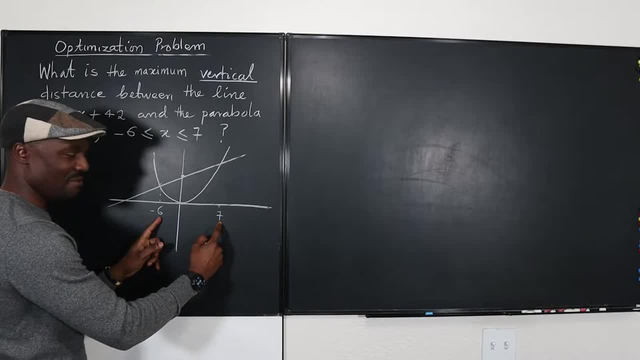 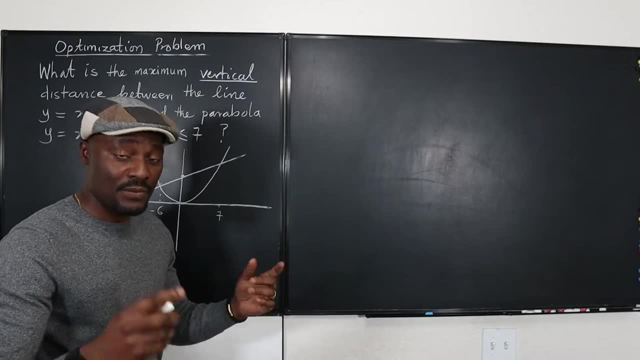 So, from here to here, where is the distance, the maximum? Just by looking, Because if you solve this, remember two functions are equal. With two functions are equal. you just have to say this is equal to this And you notice that if you say this equals this, you're going. 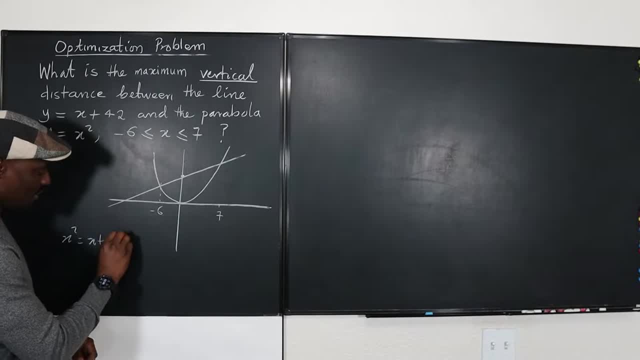 to have: x squared equals x plus 42, which says x squared minus x squared minus x plus 42.. Okay, So x squared minus x minus 42 equals zero. If you solve this quadratic equation, you're going to end up with x equals negative six or seven. That's why we're So these two. 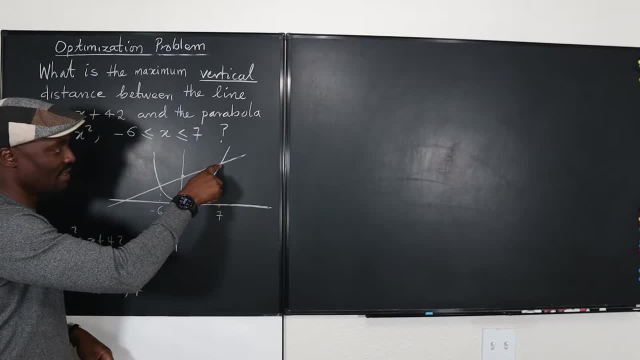 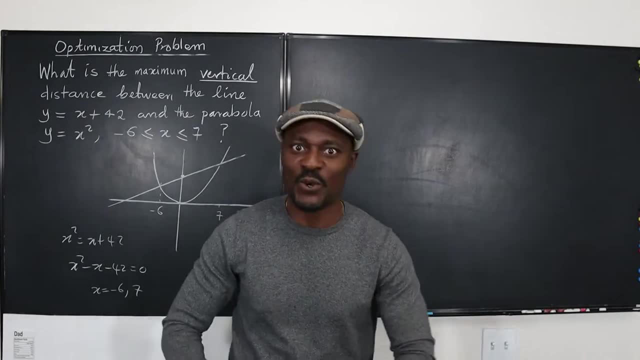 points actually. So what's the distance between the two functions at this point? Well, it's zero. What's the distance between the two functions at this point? It's zero. But let's assume you didn't know that or you didn't bother yourself, you know, with whether. 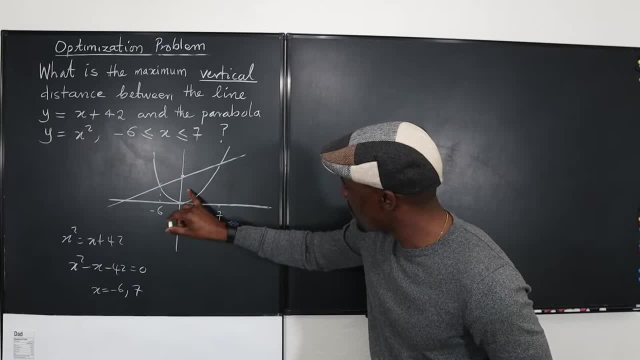 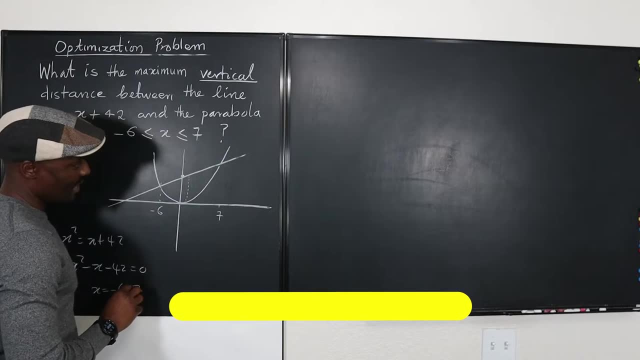 the distance here is zero. We just want to find where it is maximum. okay, I think the maximum point should be somewhere here, Somewhere here, I'm not sure. okay, But we will investigate as long as we know where the point is, Okay. So what do we need? 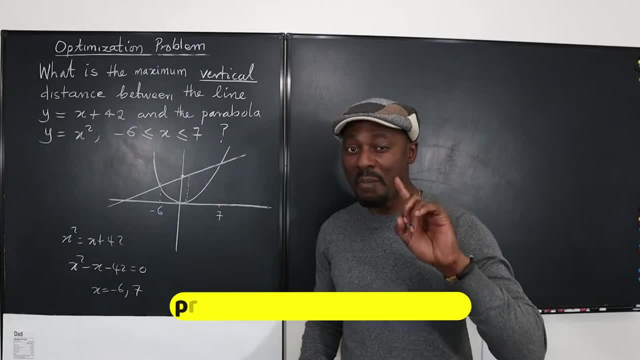 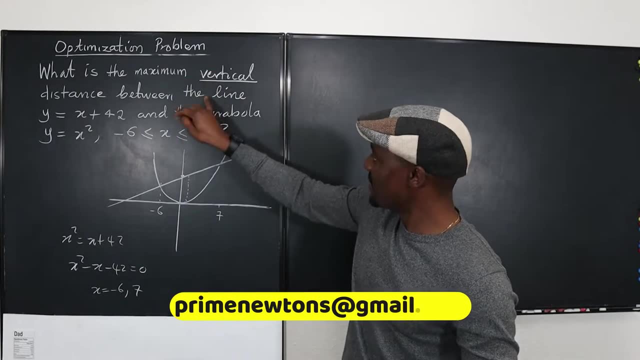 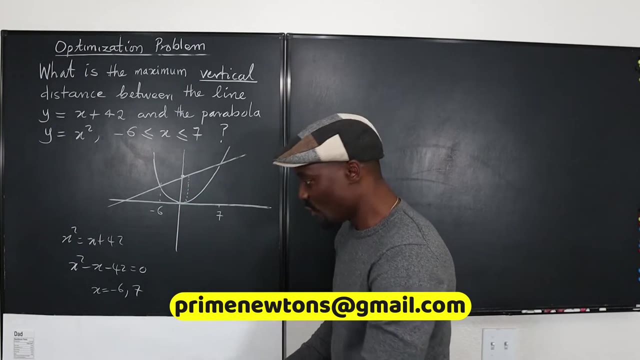 to do to find the maximum distance. Remember that Like not maximum distance, maximum vertical distance. If it's a vertical distance, it means you're not moving sideways. X is not changing, What is changing is just y. So, as you can see here, let's say it's this point. We don't know what this point is, but 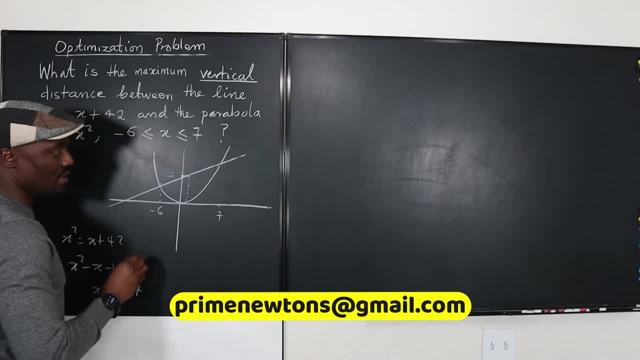 we know this point will be some y, Let's call it y1.. And this point is going to be some 2.. Let's call it y2.. And it's so obvious also that this is on the line, So this we could. 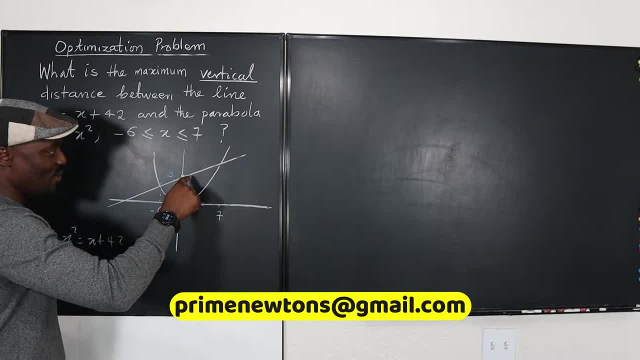 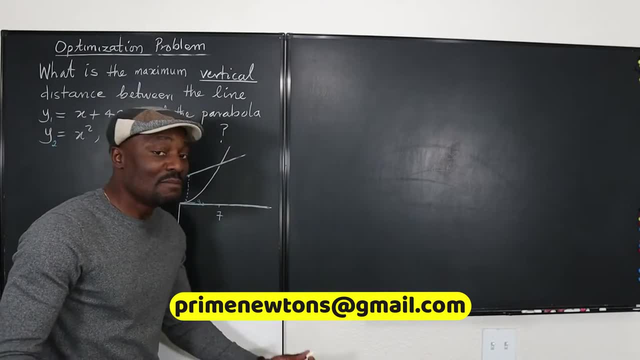 say this is our y1,, okay, And we could say this is our y2,, which is the parabola. It doesn't mean it is Correct, okay, But let's just say that's what it is, But obviously from the graph it's there. 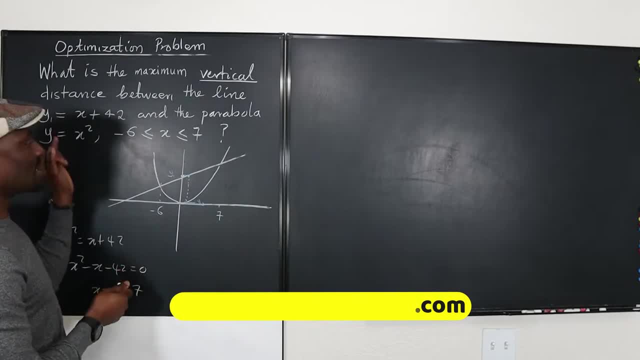 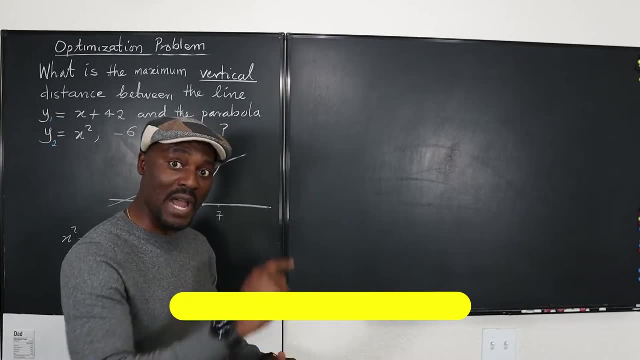 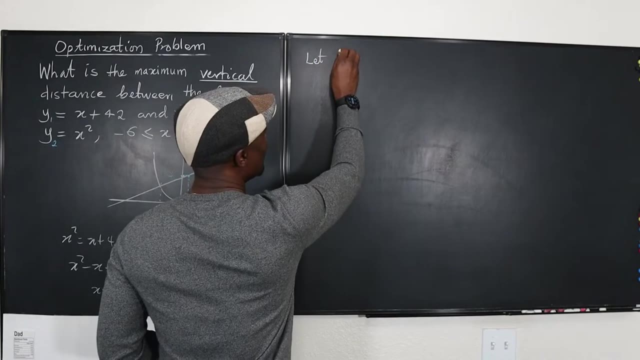 So, assuming you didn't sketch any graph, you could take this as your y1,, take this as your y2, it doesn't matter. But the vertical distance between the two functions is the difference between the two y's. So you can say: let the vertical distance, Let the vertical distance. 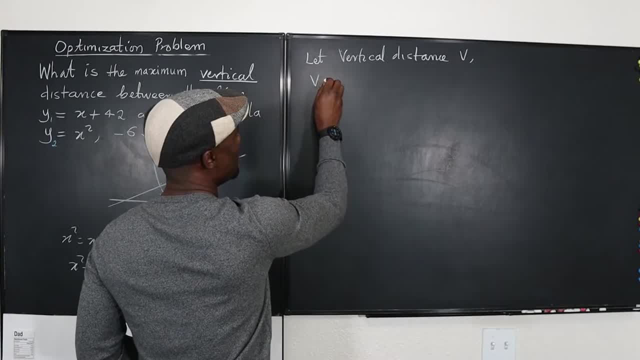 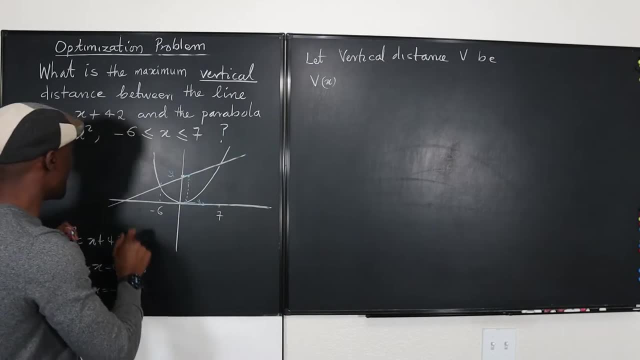 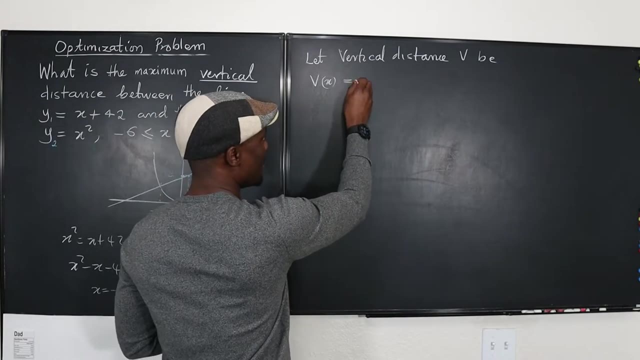 Be okay. Be such that v of x. okay, Be v of x, So v as a function of x would be. I'm going to be subtracting. Remember, when you want to find the distance from here to here, it's just y1 minus y2, okay, It would be equal to y1 minus y2, which, in this case, 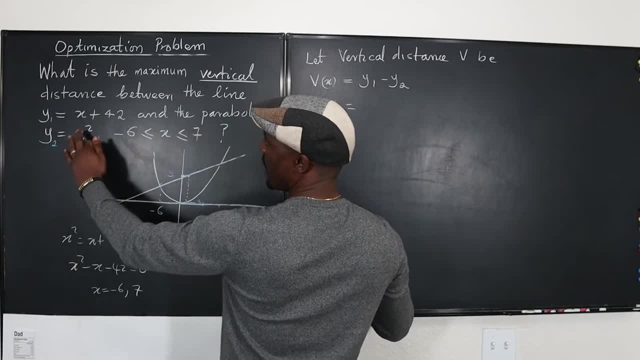 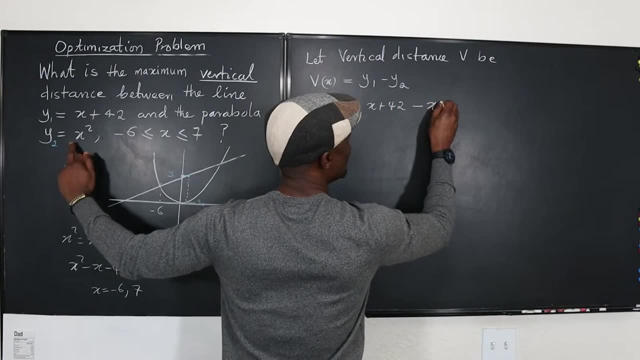 we can say: v of x is equal to What is y1?? Um, x plus 42.. x plus 42.. And what is y2? is this: So it's minus x squared. So you found a function that represents the distance between. 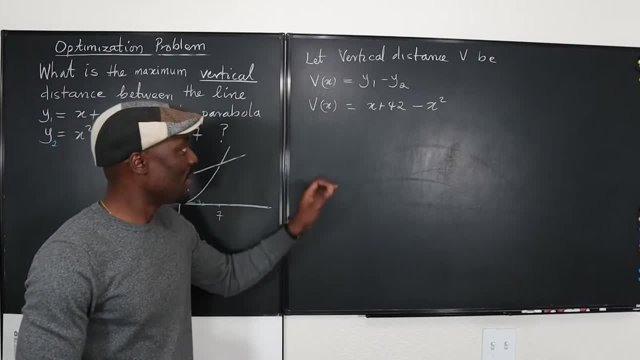 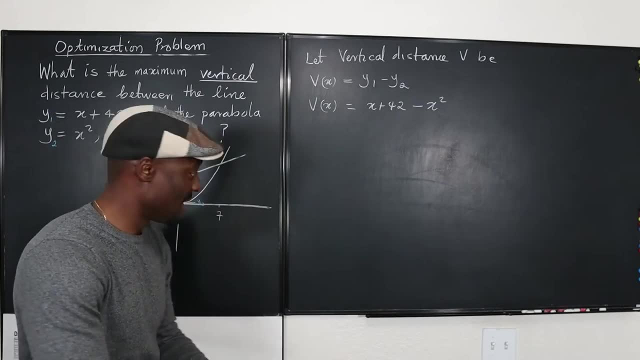 these two functions at any time. If you plug in any number here, it will tell you the distance between these two points. For example, just if you want to test, if you plug in negative six into this function, you're going to get zero because the distance between the two functions 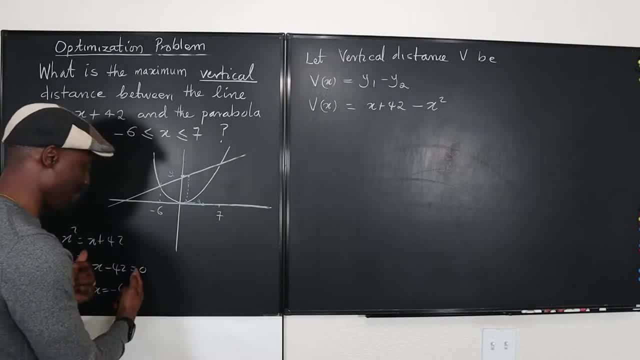 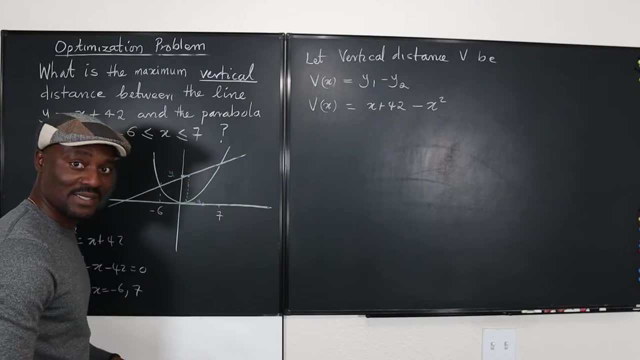 is zero. Yeah, I'm sure. Oh, yeah, it's true, because the only roots of the quadratic that we have here. So you're going to get zero. If you plug in seven, you're going to get zero, because that's the distance. So the point we're really looking for is somewhere in between, and there'll. 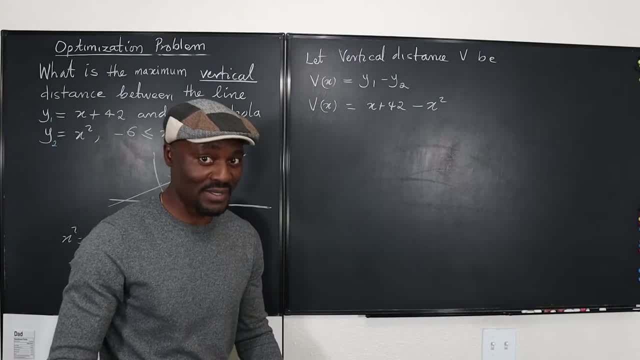 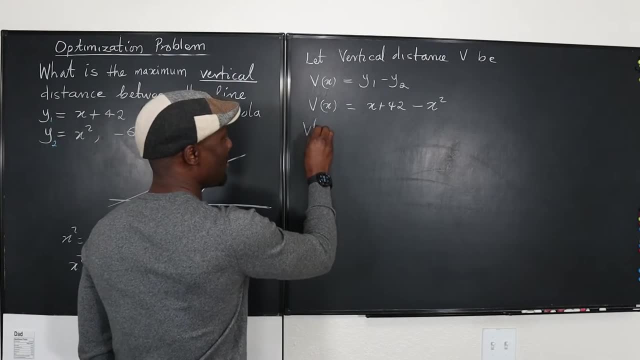 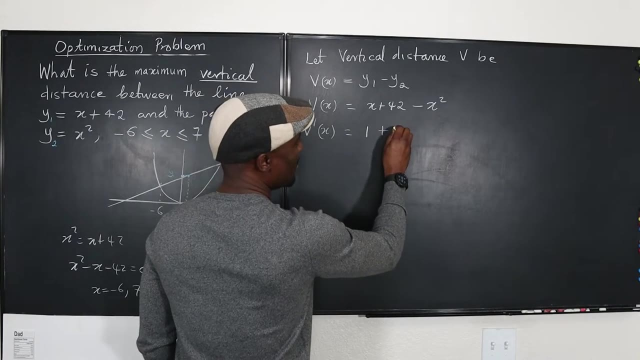 be a critical point And remember what happens at a critical point. Yes, the derivative of the function is zero. So let's take the derivative of v of x. So v prime of x is going to be the derivative of this function, which is going to be one, And this goes to zero, And this is going to 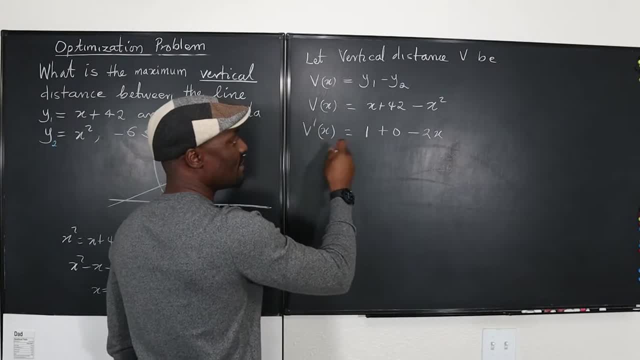 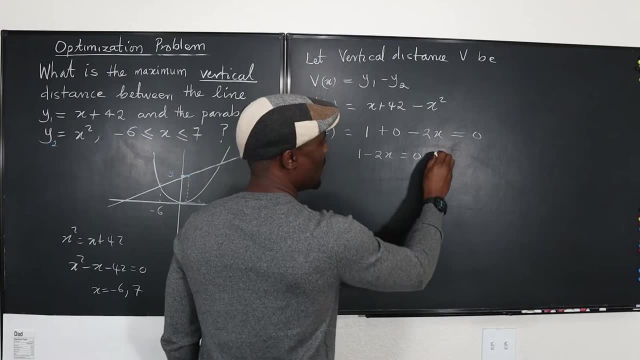 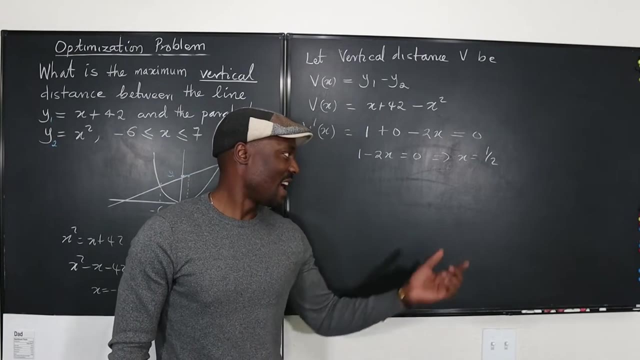 be minus two. So remember that the derivative is always equal to zero. when you take this derivative, So that means one minus two. x equals zero, which implies x is one half. So we just need to be sure that this is a maximum point, not a minimum point, because this is a critical number. So 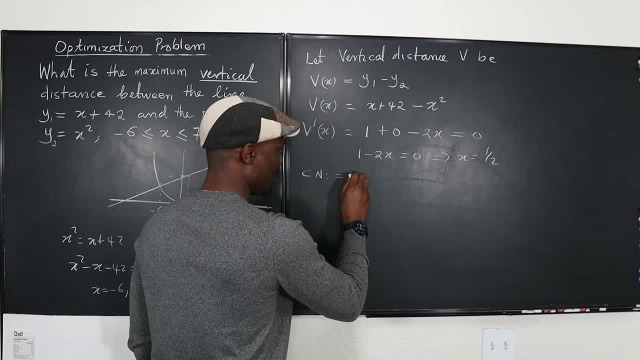 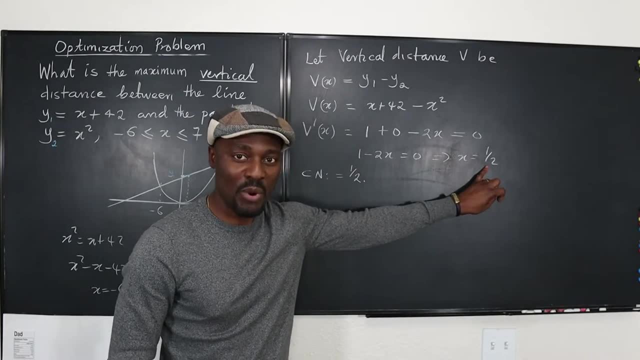 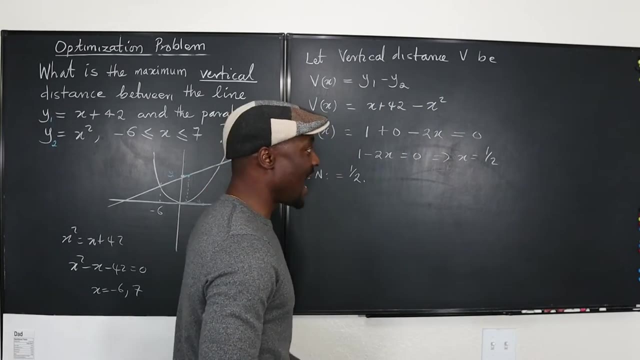 the critical number we have. critical number equals one half. Okay, there are two ways to go about this. So, again, you need to be sure that this is the point where the maximum distance occurs. You just want to do a sign chart. Okay, so two ways It is: either you take the critical number and the 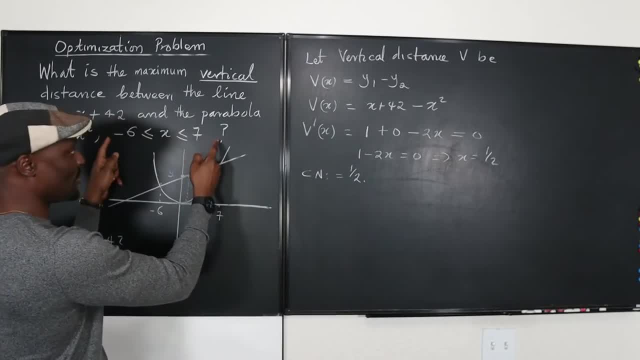 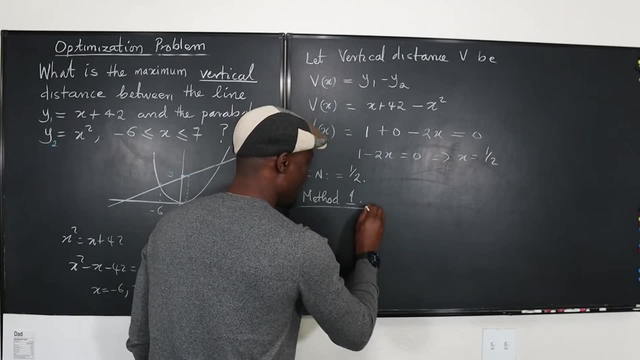 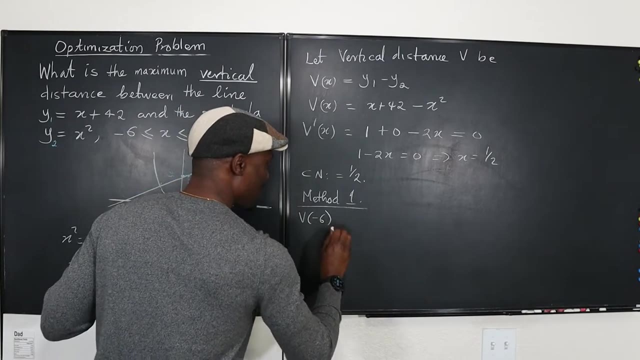 end point as method one, because you have a boundary. If you have a boundary, you could use this. Let's call this method one. Okay, so method one is you plug in the values. So you're going to say: what is v of What's the smallest number Negative six? And then you also find the next one. 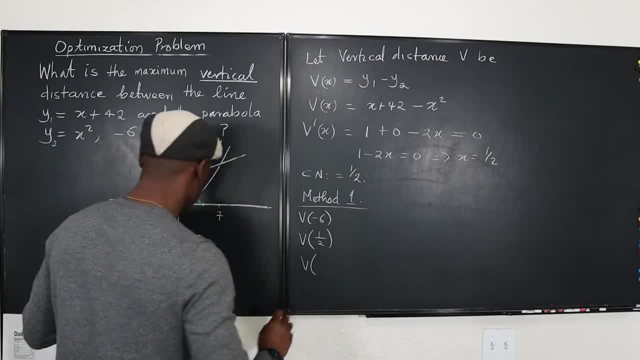 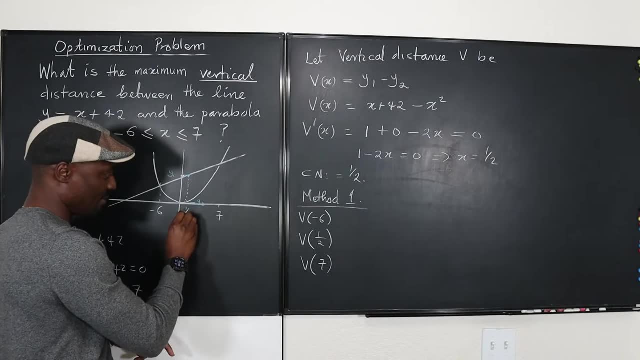 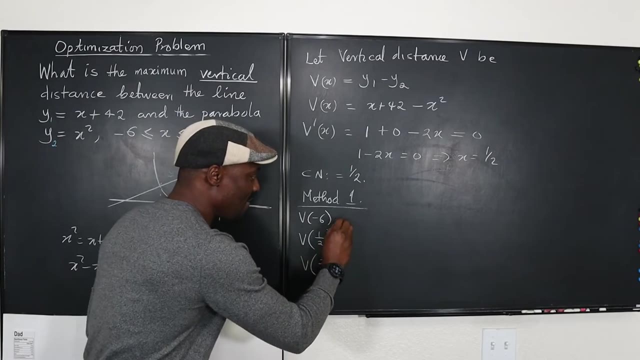 one, what is v of one half? and you say what is v of seven. you're trying to find the vertical distance at these different points. so this point is the point one half. just as we just calculated and as you can see from the graph, it is the answer. but let's show it now. if we evaluate this, 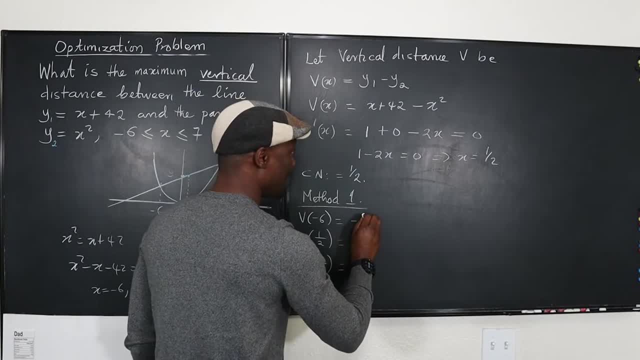 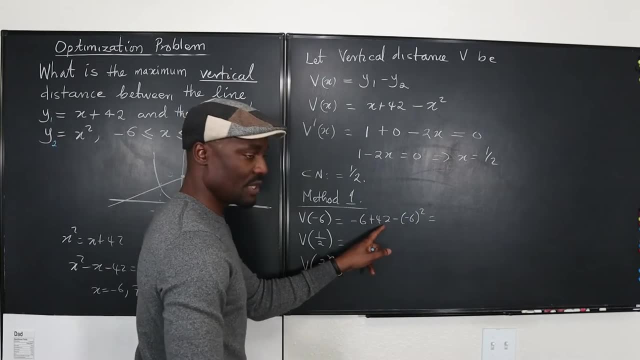 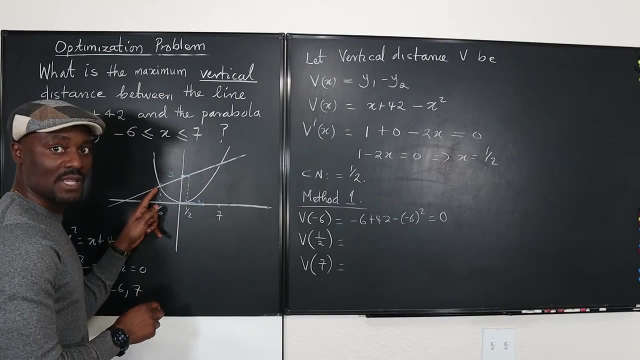 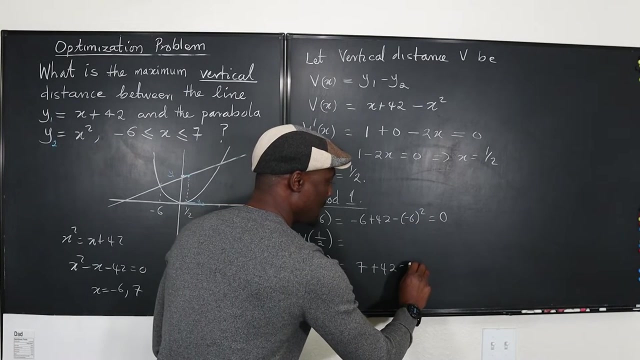 if you plug in negative 6 into this function, you're going to get negative 6 plus 42 minus negative 6 squared. this is negative 6 plus 42. that's 36, 36 minus 36. it gives you 0, which shows that we're correct. okay, there's no distance. let's do this one. let's do 7 plus 42 minus 7 squared. 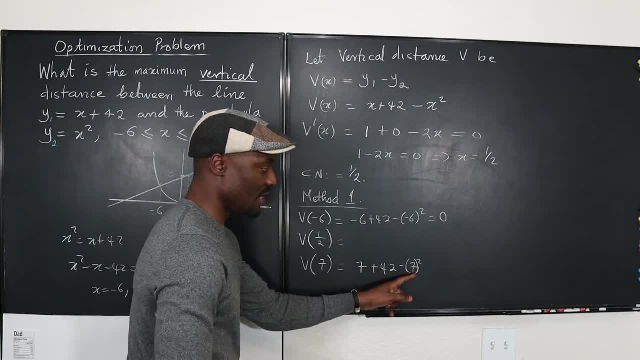 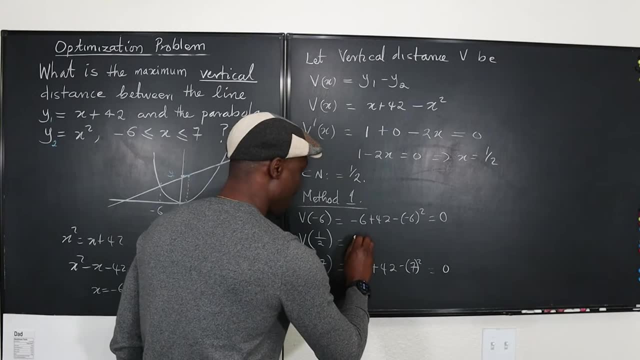 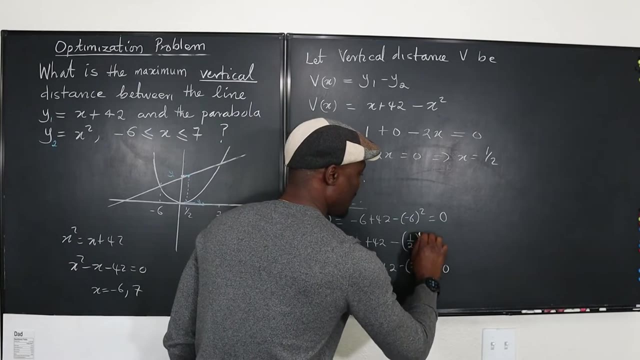 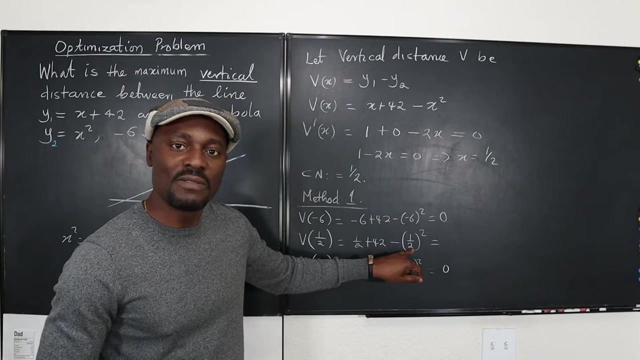 okay, this is going to be 49 minus 49. that gives you 0.. so if we go here we want to find the distance, it's going to be one half plus 42 minus one half squared. i can tell that this is 42.5, just to help myself, and this is 0.25, which is one-fourth. 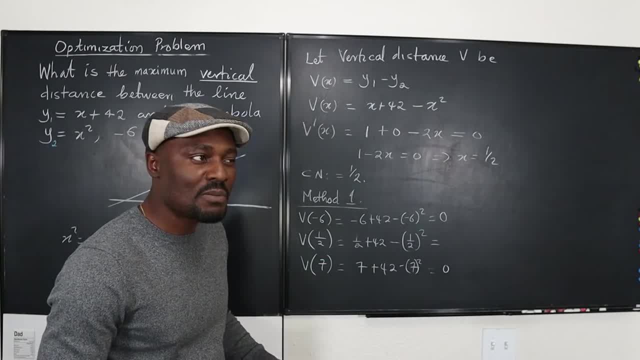 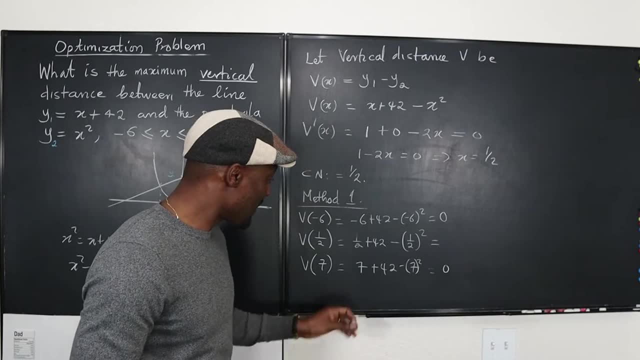 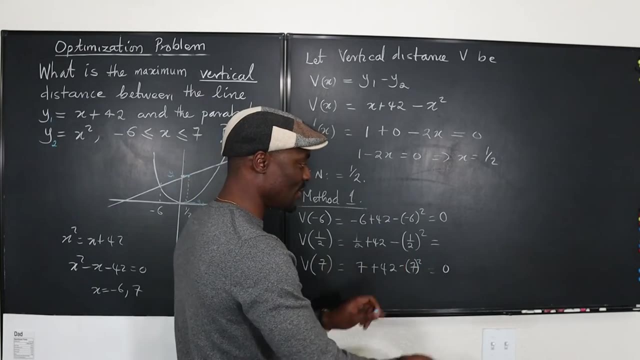 so 42.5 minus 0.25 is going to be 41.2. oh, what is that? okay, so this is one half minus one-fourth is going to be one-fourth, so it's 42, one-fourth so it's going. 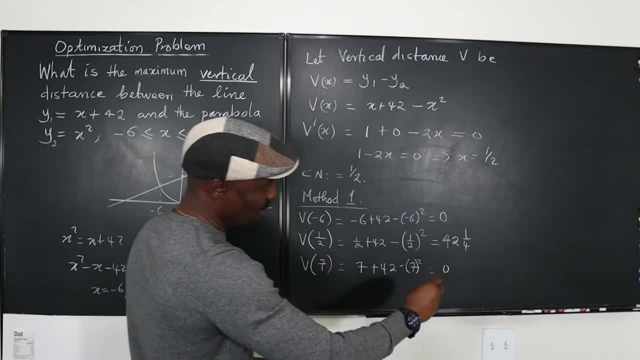 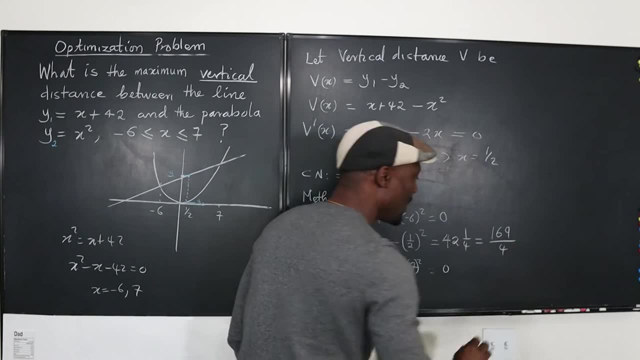 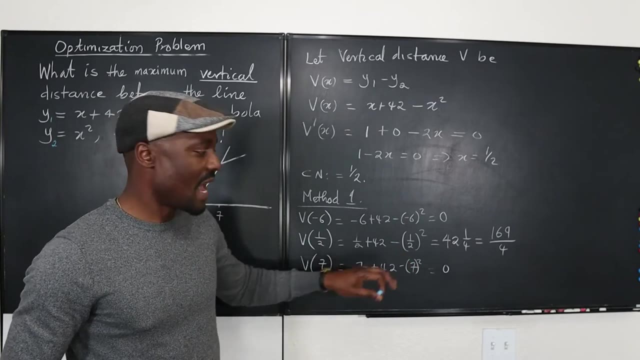 to be 42 and one-fourth, which will translate to what is four times 42. it's 168 plus 169, 169 over four. so, as you can see, this is the maximum distance. okay, the sign chart is just to help you confirm that you don't have to do these two. um, you just need to be sure that this is a maximum point. 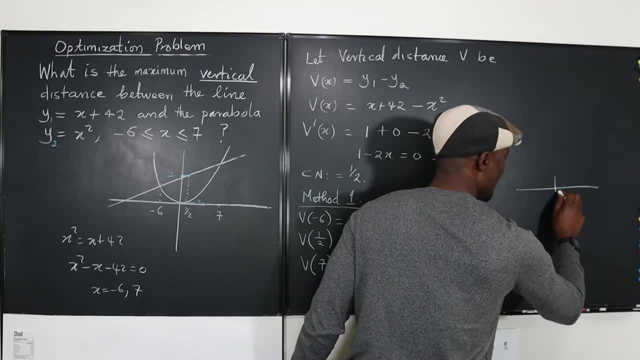 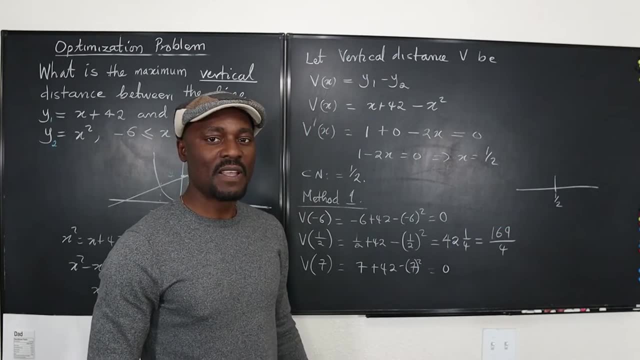 and you'll get it. and what the sign chart just does is that you have to get the maximum distance, is that you tell yourself: this is one half and i'm going to try out all numbers, um that are left of one half and see if my slope is going to be positive or negative. remember this. 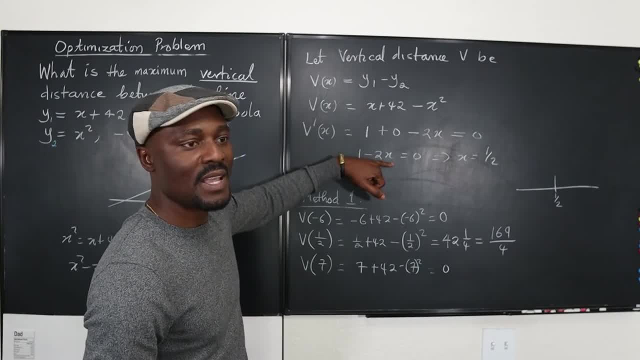 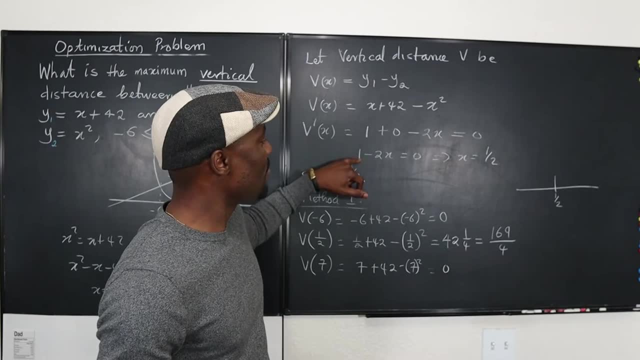 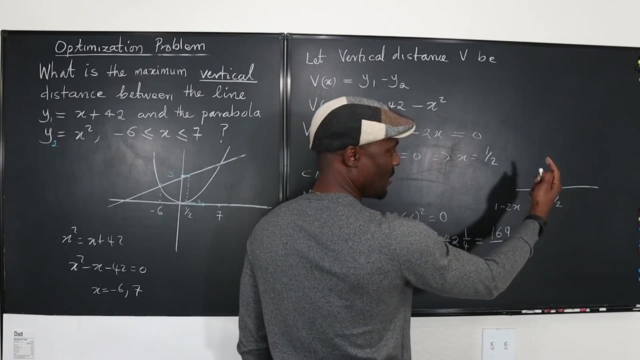 is the equation of the slope. it's 1 minus 2x. okay, so if i pick any number that's less than one half, say negative one, put negative one here, what would you have? you're gonna have one minus. see, one minus two x. if you put negative one here or anything less, zero even. 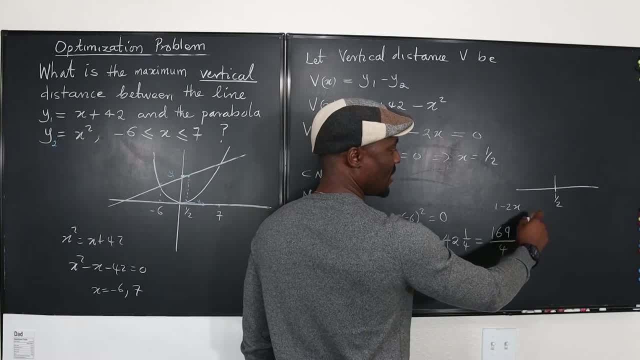 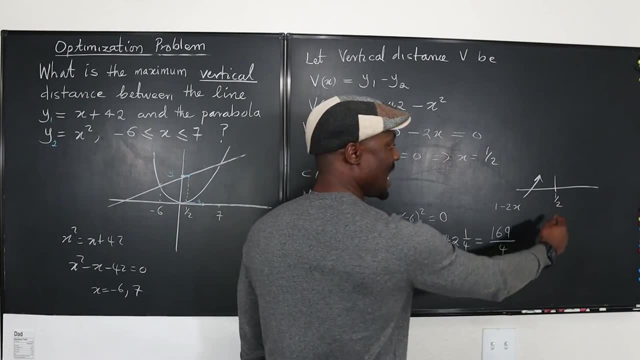 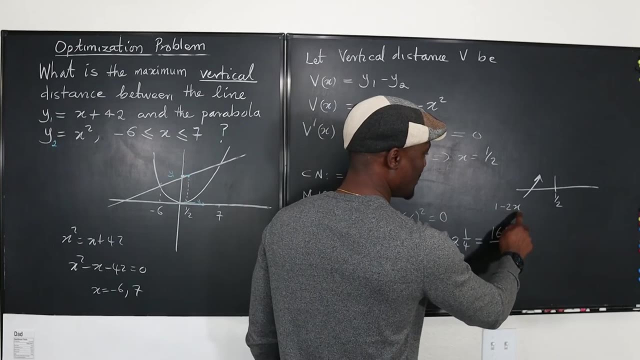 if you put zero here, this is gonna be one minus zero. so no, zero is not positive. okay, oh, one minus zero is one positive. so it goes this way. and then if you pick any number greater than one half, so if let's pick um one, if you put one here, one minus two will be negative one, it's going to be a. 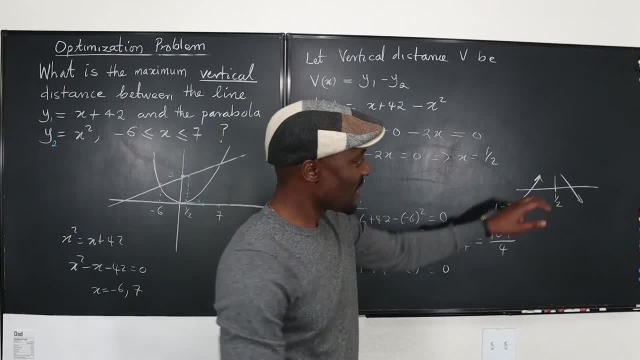 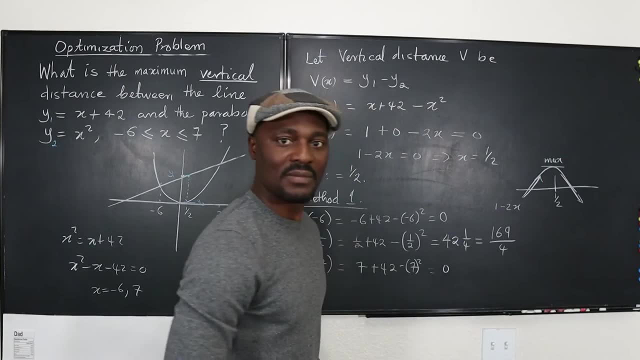 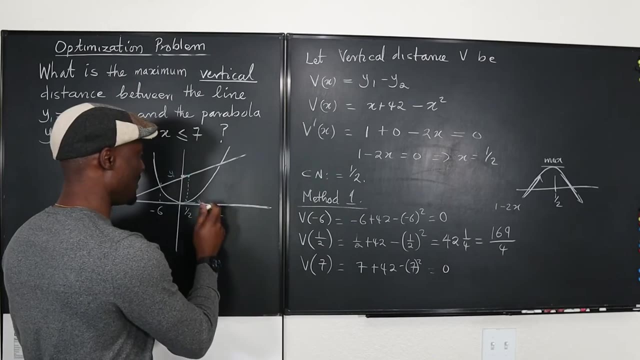 negative slope. so, as you can see here, this graph goes like this and comes back down. so this definitely is a maximum. okay, it's a maximum, so it's a local maximum and it's also the absolute maximum for this range or this interval that we have here. so we can say: we know that the maximum occurs when x is one half. 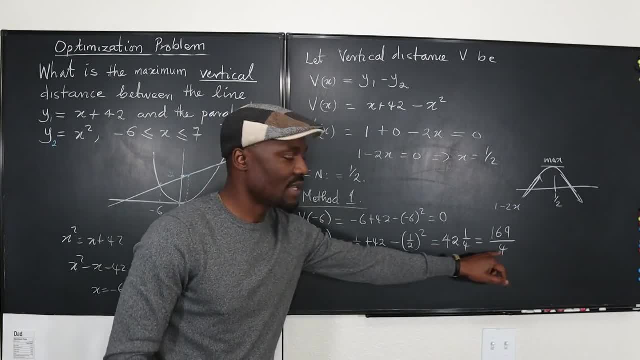 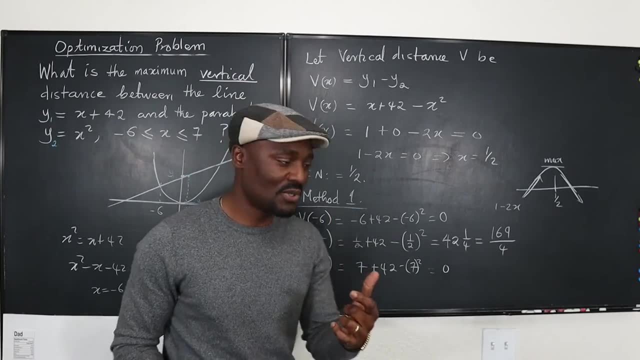 and then you go plug in one half into the function and you're going to get this answer. okay, but my recommendation: every time you're given end points and you you can find the critical numbers, just plug in the numbers and see which one gives you the biggest answer and that's your maximum. i hope. 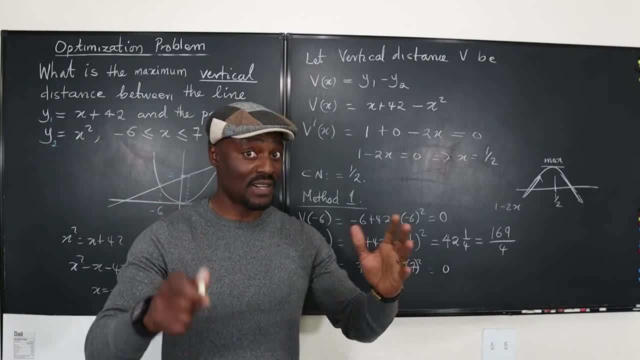 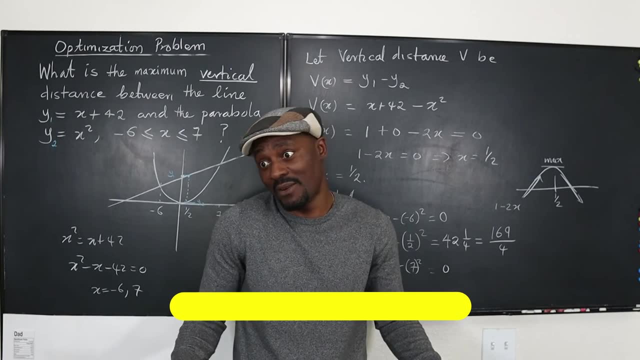 this video was helpful if it did help you give it a like, share and be subscribed. if you're not, most of my subscribers are not subscribed. i don't know what you're doing, why, but you got to tell me in the comment. in the comment section, tell me why you're not subscribed. if you're watching this video and you 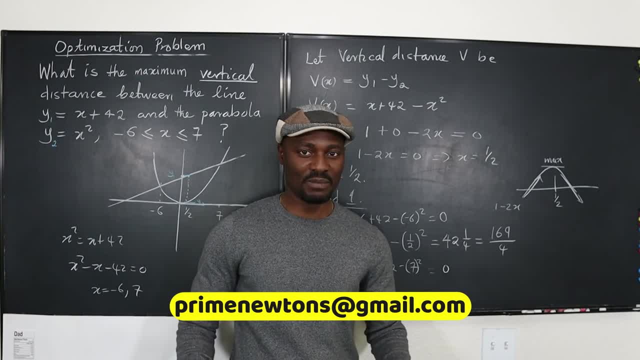 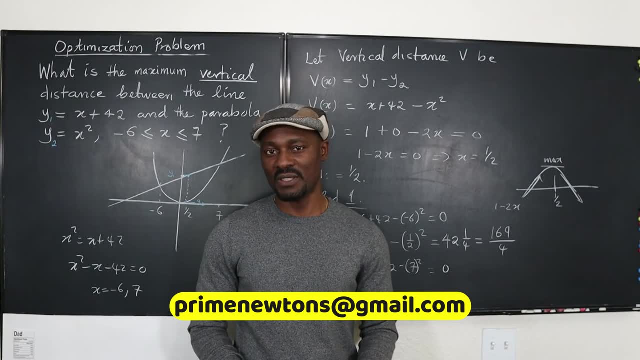 find it helpful just before i go. if you need any help with math tutoring or whatever you need to do, just get in touch with me. send me an email: primeneutons, gmailcom. i could do a zoom with you. you, if you're far away from Los Angeles, If you live in Los Angeles and you prefer one-on-one. 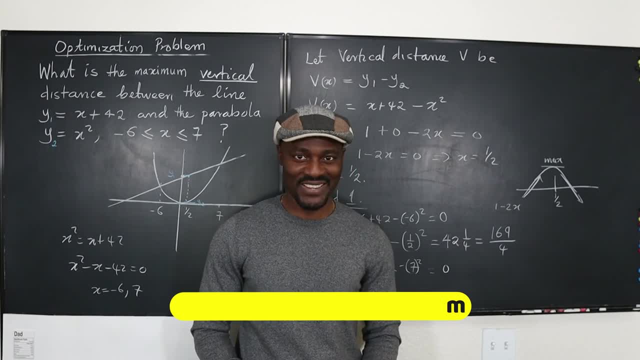 with me. I'll be available to help you too. See you in the next video. Don't stop learning. Those who stop learning have stopped living. Bye-bye.